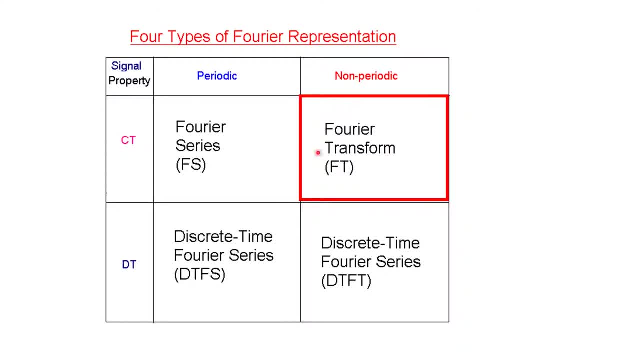 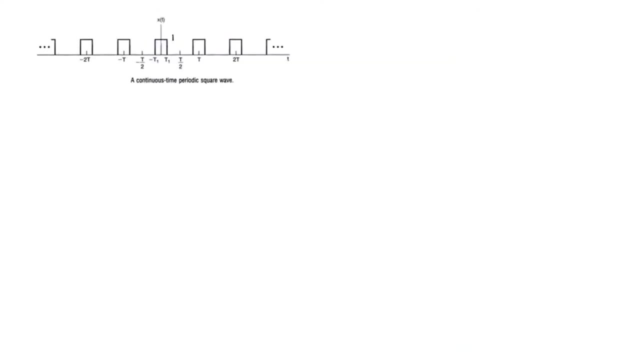 Fourier transform. So in this video we will be studying Fourier transform, where the signal is continuous time but it is non-periodic or aperiodic. Now, before we go to the actual derivation, let us recall or recap from the Fourier series We had a periodic square wave signal and over one period between here to here we can. 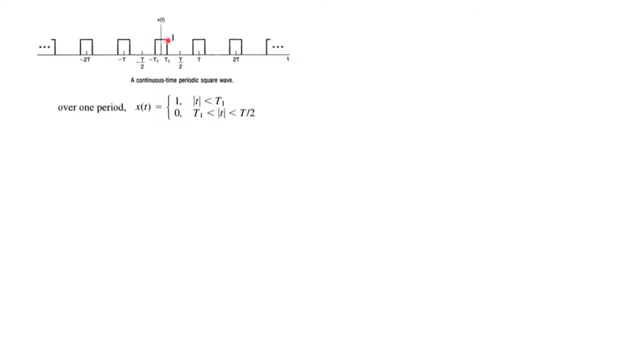 say that xt is 1, 1.. For t between minus 1 and plus 1.. So mod of t is less than t1 and 0 here and here for t between t1 and ty2.. So this range and this range, and in chapter three for the 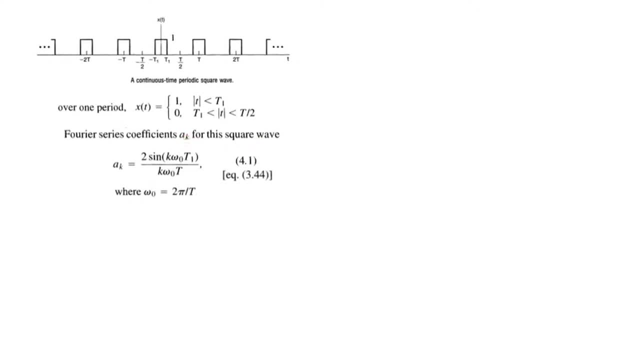 signal. we had found out that the Fourier coefficient, a, k, is given by this formula, where we know that omega naught is 2 pi t, So this equation is actually 3.44 from chapter number 3, and if we multiply by t or we take t on the left hand side, and also we replace k omega by omega, 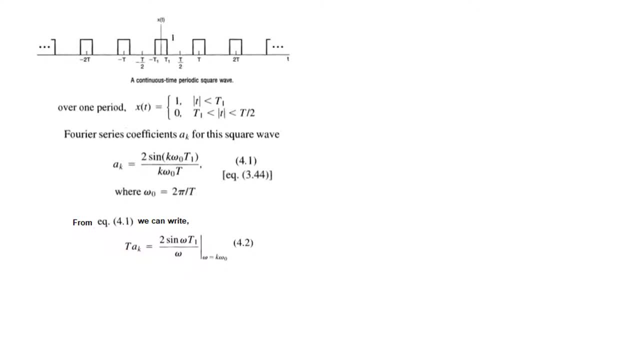 then we get equation 4.2, which is like this, that is t a, k is equal to 2 sin omega, t, 1 over omega. Now, if you notice here, So omega is equal to k, omega naught where k is an integer but omega is not an integer. 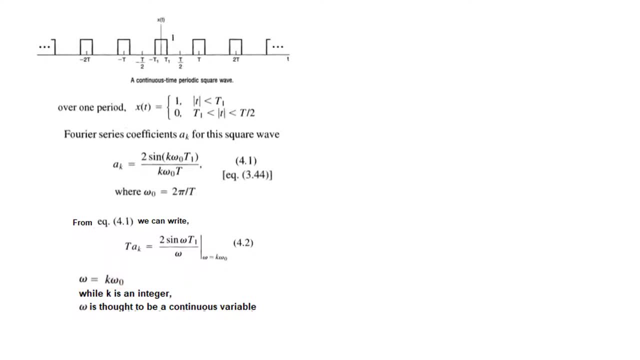 because omega naught could have any value, any fraction, and that multiplied by an integer will give you a fractional value. So omega is considered to be a continuous variable, that is, it had value at every place. Now let us see this figure. this was the representation of the coefficient a, k. 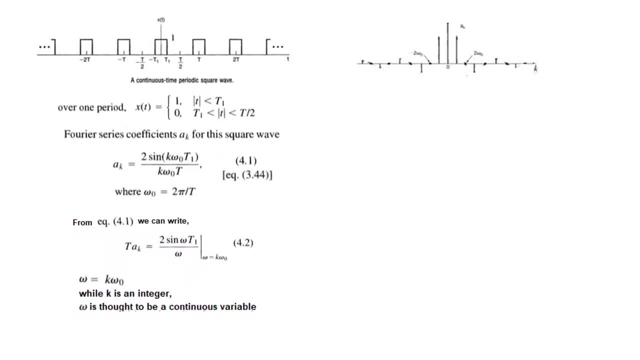 So it is represented like this: a zero, a 1, a 2,, a 3,, etcetera, and the axis was in terms of k. Alright, Okay, Uh, But when we talk of this thing, sin omega, t, 1 over omega. so this is a sinusoidal function. 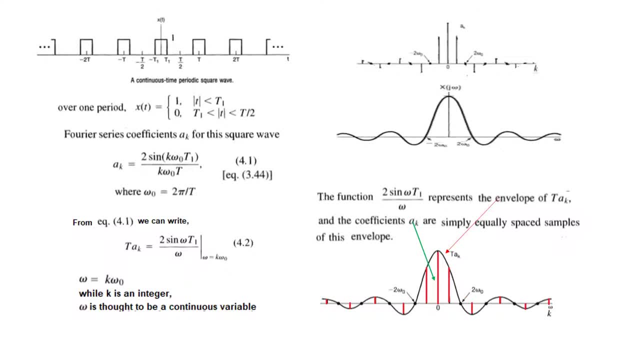 a continuous function and its amplitude will depend on, or the amplitude is decreasing gradually, you can see. So the sinusoidal function's amplitude will also decrease. So this is the representation of T a k. this function is T a k, or we can say that: 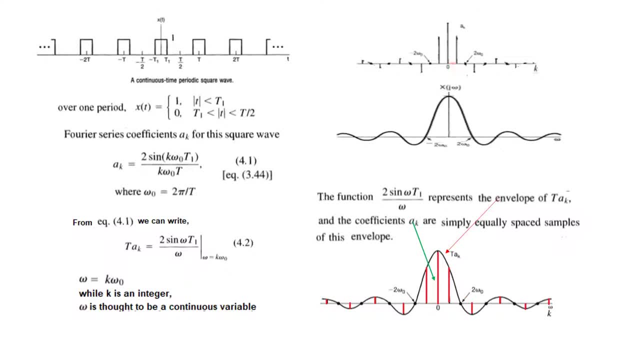 this continuous function which we can see. we have combined both of them here. So here the top line is called the envelope. This is the envelope of T a k and these lines, which can be thought of as sampling of this continuous signal, they actually represent. 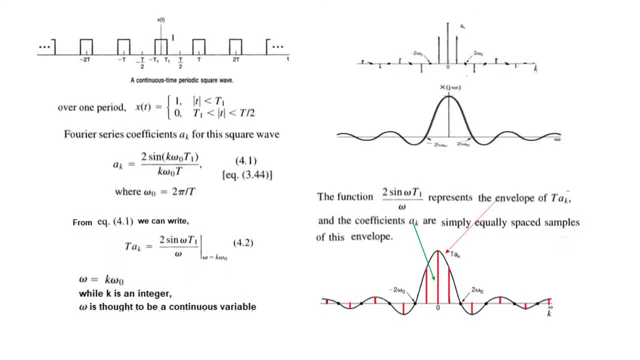 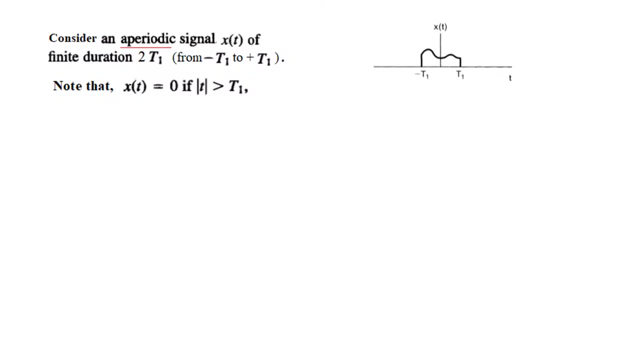 the Fourier coefficient a, k, and the spacing between them is actually omega naught. Okay, now we come to the actual derivation. We consider an aperiodic signal expression, X, t, of finite duration. duration is from 0 to T 1 and 0 to minus T 1.. So duration is 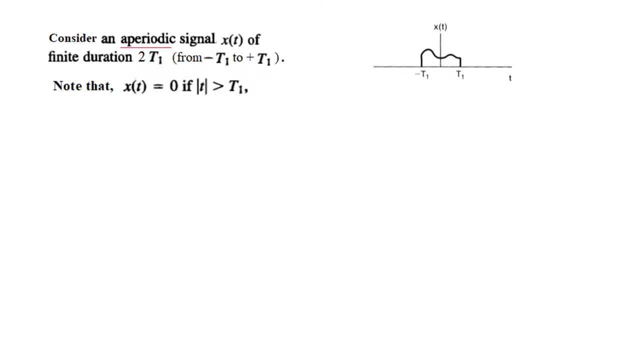 2 T 1, from minus T 1 to plus T 1, and note that X t is 0 for T greater than T 1.. So in this range X t is 0.. And now from this aperiodic signal expression we can say that the Fourier coefficient of 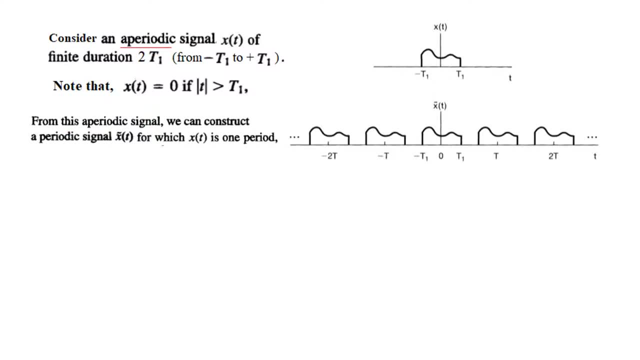 T a k is 0.. So this is the periodic signal, This one. we can construct a periodic signal X bar t, for which X, t is one period. So what we are doing, we are just duplicating this, paste here, paste here, paste here. so paste here, paste here. So this is now aperiodic. 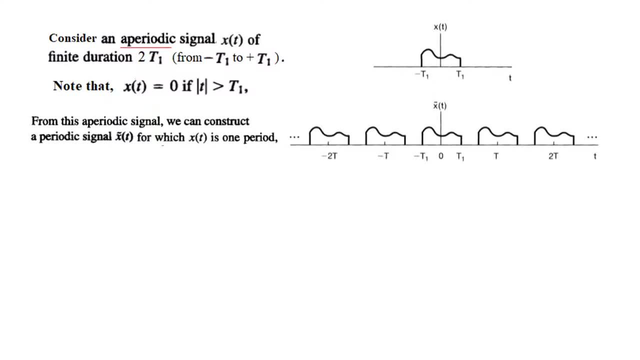 signal. And the key point to remember is the periodic that for this duration, that is, from t by 2, minus t by 2 to plus t by 2, they are same. x t and x t bar are same. Now as we choose the period t to be larger, 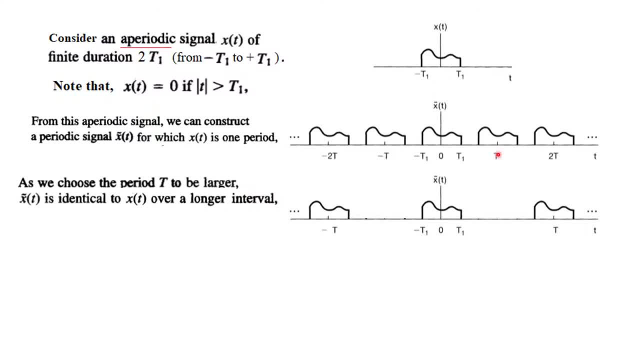 so earlier this was the time period. So if we increase the time period, so let us say, it becomes like this: So this spreading more x bar t is identical to x t over a longer interval. Now, since this is all the way, 0, so we can say that it is up to this, up to 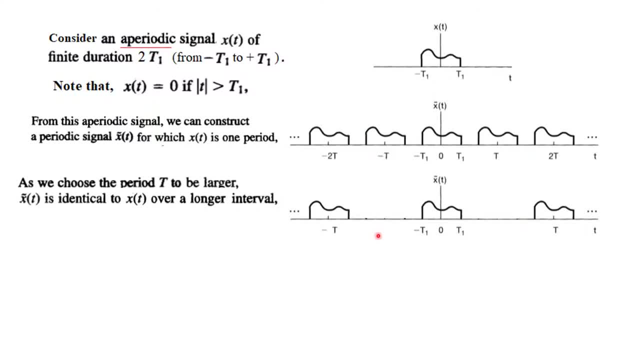 this point: x t and x t bar. So x t and x t bar are same. And now, if we extend this t to infinity, so this vanishes, this vanishes or goes beyond infinity. So as t becomes infinity, we can say that x bar. 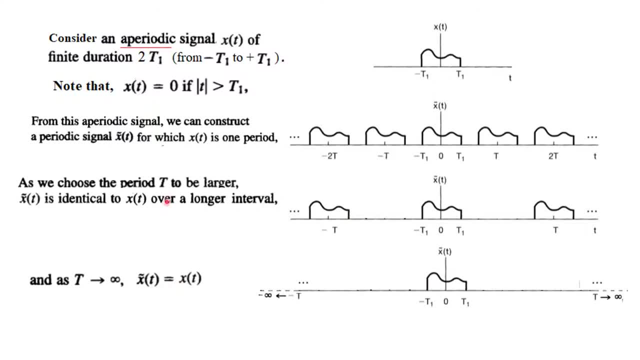 t is equal to x t, So this was x bar. we have just moved it to infinity, So we can say now that these two are same, So t becomes infinity, or the time period becomes infinity. x bar, t is equal to x- t, So this: 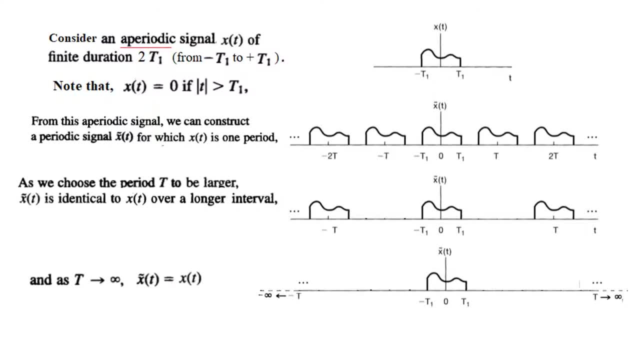 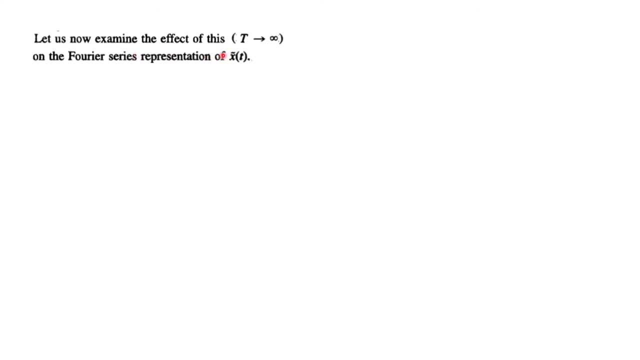 is very important conclusion that we have to keep in mind. ok, now let us examine the effect of this t tending to infinity on the Fourier series representation of the function x bar t. If you recall from chapter number 3 for the periodic square wave signal, We had these two equation for the Fourier series. one is: 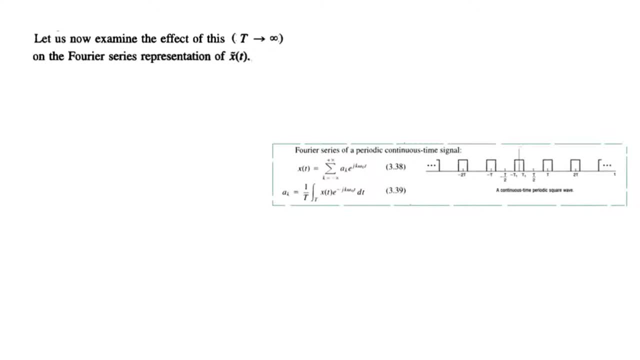 called the analysis equation and another is called the synthesis equation. So in our case, since x, t is also periodic, So we will have a similar equation. Now compare these two. Since the signal is x bar t, so we will write x bar t. summation: summation: a, k, a, k, e, power, j, k. 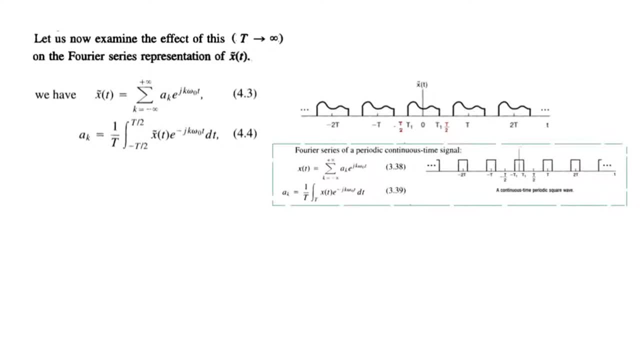 omega t. So exactly same. Similarly, the Fourier coefficient a, k, a, k, 1 over t, 1 over t, here the integral over the time period t. and we are writing instead of that from minus t by 2 to t by 2.. It is the same thing. And then the signal x, t. our signal here is: 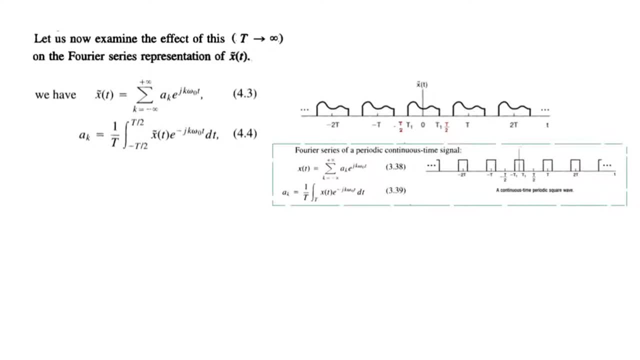 x bar t e minus j k a t t. Ok Now also: we discussed earlier that for t between t plus 2 and t minus 2- that is signal from my t minus 2 to t plus 2, x bar t and x t are same, So x bar t is equal to x t for mod t less than t by 2.. And therefore 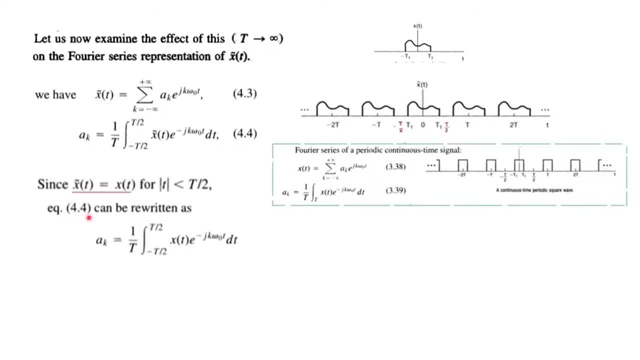 this equation, 4 by 4, we can write a k 1 over t integral same. We are just replacing x bar t with x t because they are same within this range And also since x t is 0 outside this interval. So if you remember, see this. 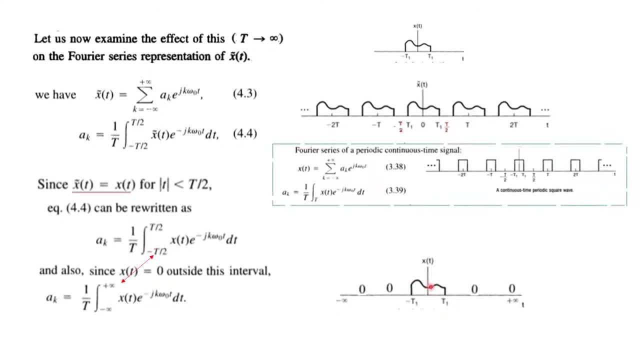 diagram. here The signal is present only up to t 1 and beyond t 1 up to infinity. So it is 0 outside t 1 through t 2.. Yeah, And therefore this level we can extend up to negative infinity and plus infinity, because 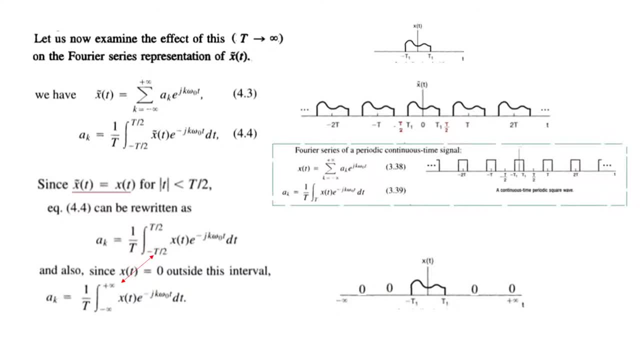 the signal is 0 outside this. So it is the same thing whether you write this or you write this. But to make it more generalized, we are now extending the limit from minus infinity to plus infinity, Thank you. And so button where we draw it from the link point. 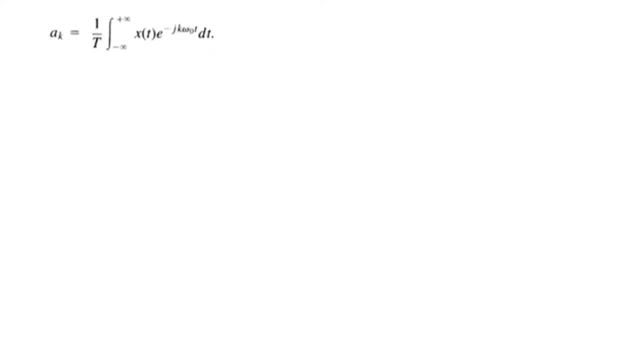 Yeah, Okay, so we had found out the Fourier coefficient, a k, by this formula, And if we take t on the left hand side, it will become t. a k is equal to integral x. t e raised to the power j, q, omega, naught t. 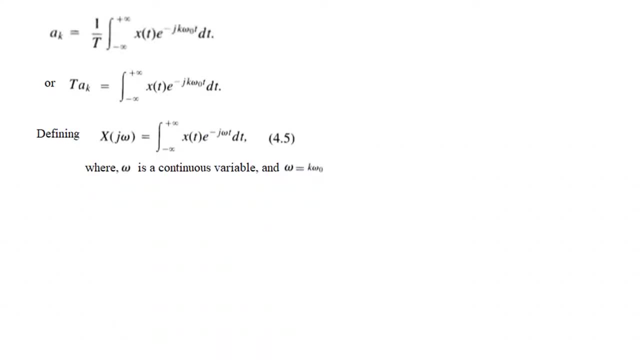 And if we define a variable, x, j, omega, keeping on the same line, just changing: k omega naught with omega. So x, j omega is integral, x, t, e raised to the power, j omega naught t, dt And omega is equal to q omega. 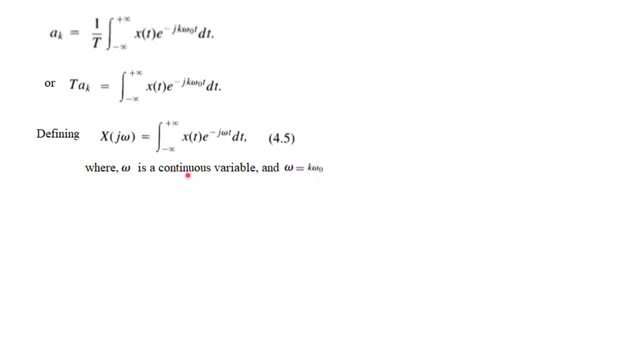 And also omega is now a continuous variable because omega can have any value. So we can say that t a k is equal to x, j omega for omega is equal to q omega naught, or at omega is equal to q omega naught. 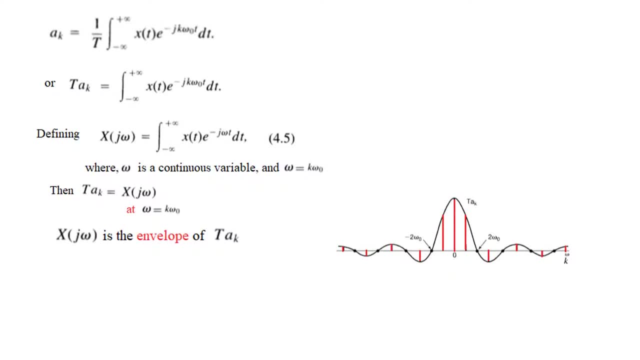 And therefore, if we see this plot, this is the envelope of t a k and we can say that this is x j omega. So x j omega is equal to t a k. x j omega is the envelope of t a k. 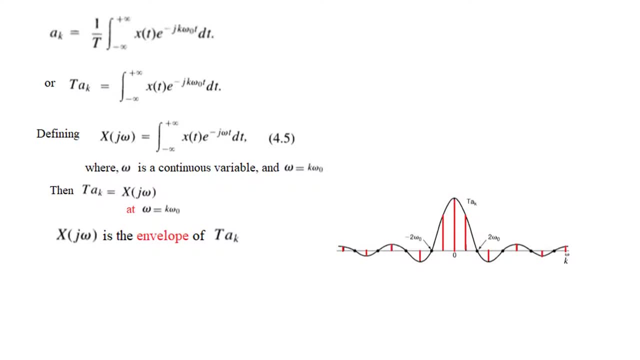 Okay. so, because This is now a continuous sinusoidal signal with amplitude gradually reducing, From this relation we can also write: x, j, k omega naught is equal to integral, just replacing omega by k omega naught. And this we are doing because we want to write. 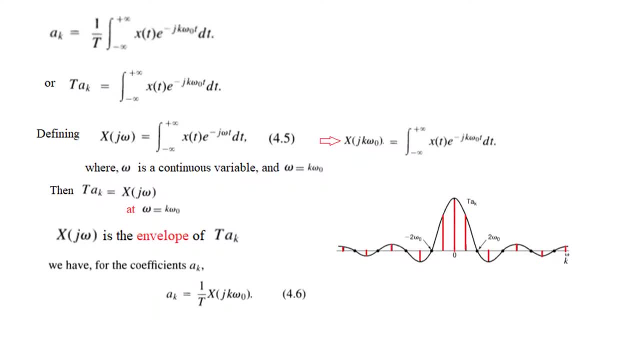 Okay, a k in the form 1 over t, 1 over t and this whole term. this whole term is now equal to x j k omega. So we are replacing that by x j k omega naught. So this is another form of representing the coefficients. a k. 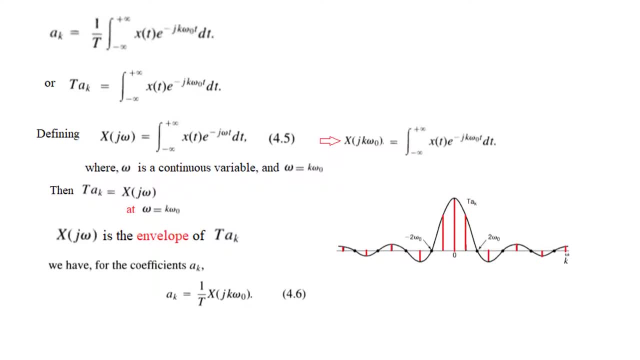 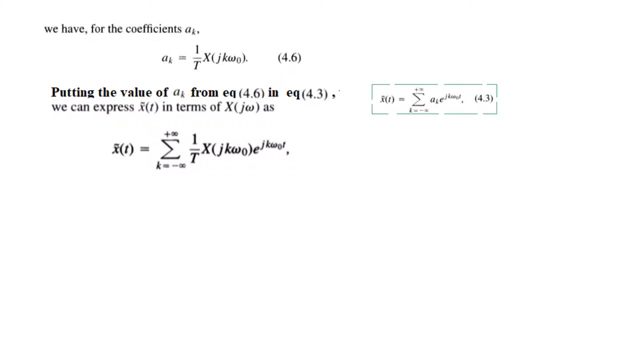 And these are those coefficients Or the samples. So we had this equation for the coefficient, Now putting the value of a k from equation 4.6 in equation 4.3, which was for x bar t, in the summation form. 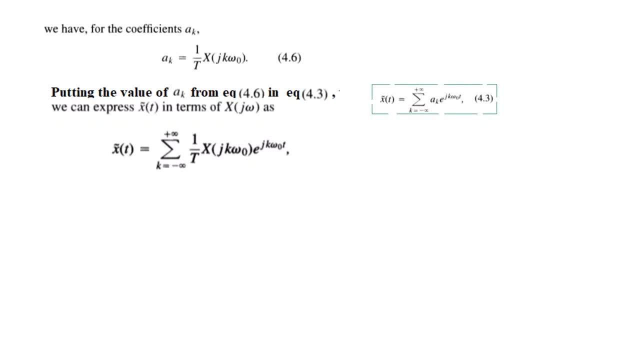 So our x bar t will now become 1 over t. x j k omega naught e. j k omega naught t. We just compare these two, Putting the value of a k, This whole, we are putting or replacing a k. 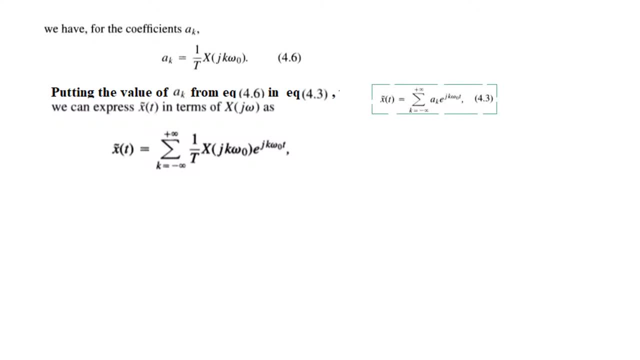 So this is our new equation for x bar t. Now we know that 2 pi t is Omega, or t is 2 pi omega, or 1 over t is omega naught over 2 pi. So 1 over t we replace by omega naught over 2 pi. 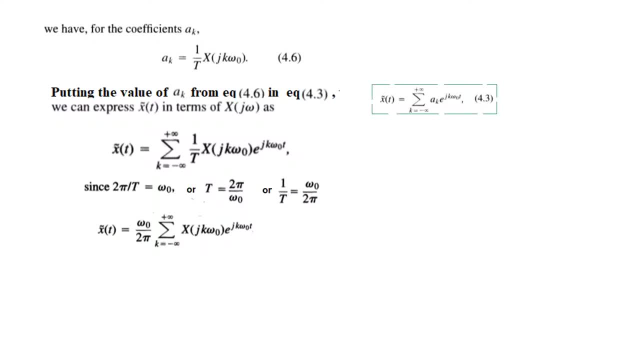 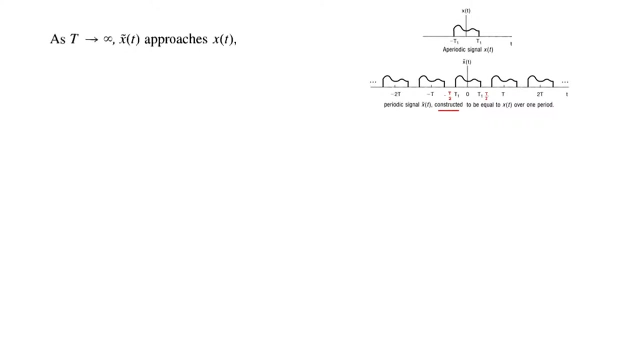 So x bar t becomes in this form. Next we move omega to the right-hand side. It comes here. So we get a new equation, equation 4.7.. Now we have seen earlier that, as t is tending to infinity or becoming infinity, x bar t is equal to xt. 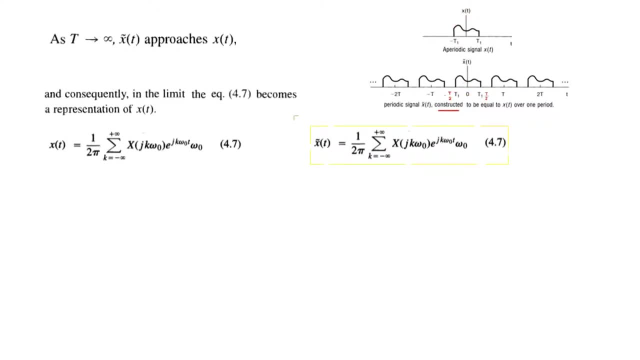 And consequently in the limit of equation 4.7,. this is equation 4.7.. Limit is from Okay, Okay, Minus infinity to plus infinity. The equation 4.7 becomes a representation of xt. What it is meaning that we can replace x bar t with xt within this limit when t is approaching infinity. 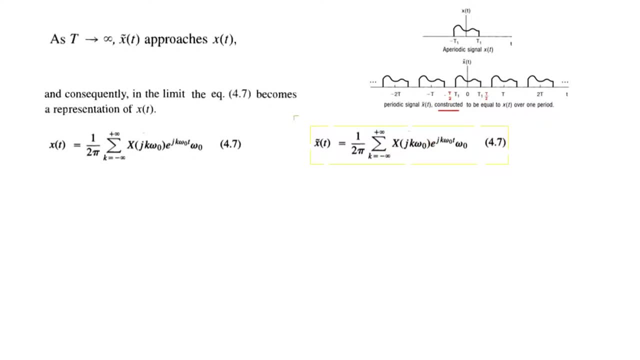 In the equation 4.7, we have just replaced x bar t with xt. Now, this is This is our 4.7 equation. now, Furthermore, as t becomes infinity, omega naught becomes 0, because we know, omega naught from here is 2 pi over t. 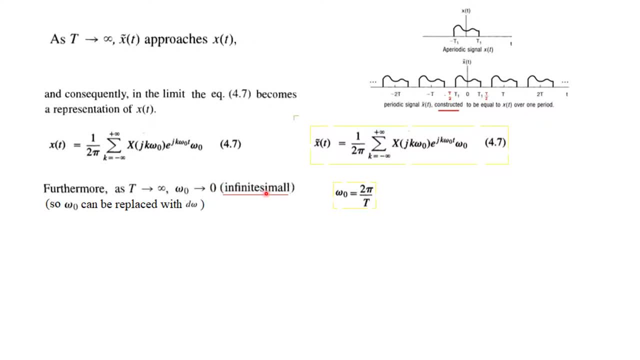 So omega naught is becoming 0 or infinitely small. So omega naught can be replaced by d omega. We know that in integration we use d omega To represent very, very small quantity. So omega naught in this equation can be replaced by d omega. 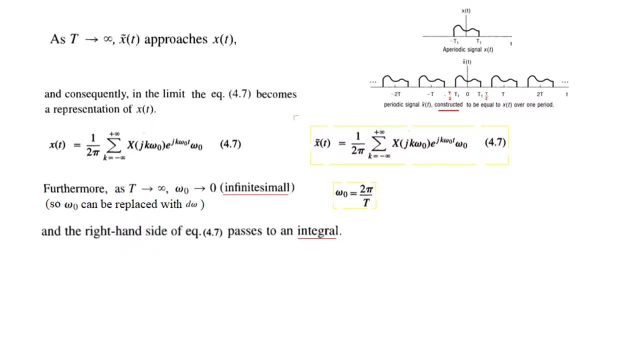 And why we want this? Because the equation on the right-hand side, this equation is now passing to an integral, or becoming an integral instead of summation, Because this term is now so small And you know the concept of summation and integral. 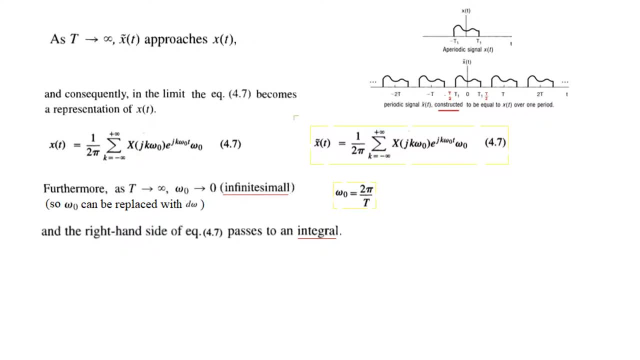 When the quantities are of reasonable size, like numbers 1 plus 2 plus 3 plus 4,, then we use the summation equation. But when the numbers become very, very small, that is, the difference becomes very small, like 1.001,, 1.002, 1.003.. 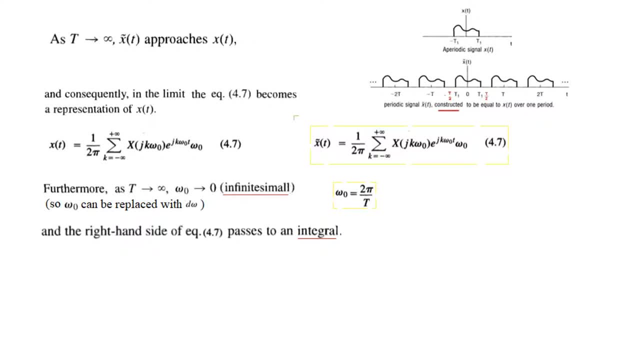 And then we, instead of using summation, we use integral. So same logic here: Since omega naught is becoming very, very small, so the multiplication is also becoming very small, And therefore, instead of summation, we will now use the integral. 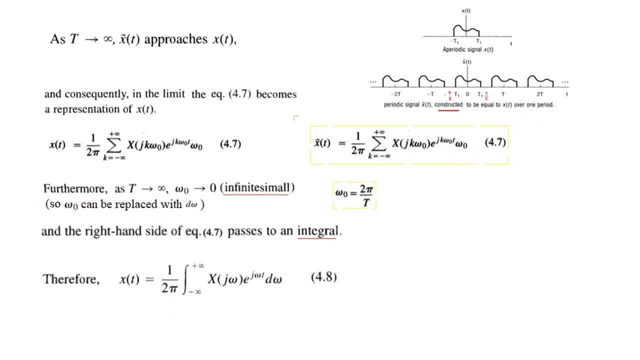 So this equation now changes to 1 over 2 pi, Summation sign, changes to integral sign And rest of the things: xjk omega, k omega is now j omega And ejk omega naught t is ej omega t. 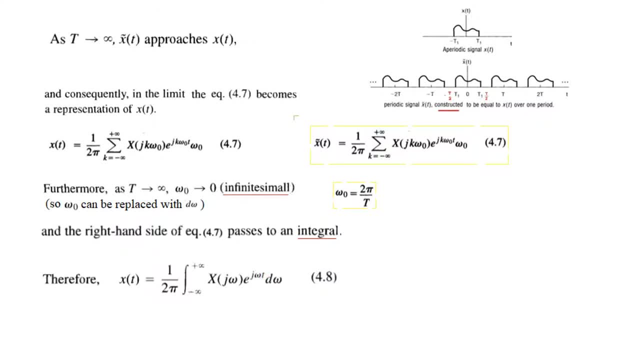 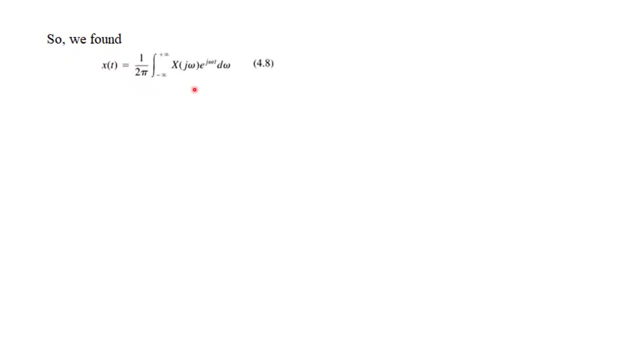 And omega naught is dw. So in the previous slide we found out xt to be in this form, which is equation 4.8.. We had also found out xj, omega, from equation 4.5, which is reproduced here as equation 4.5. 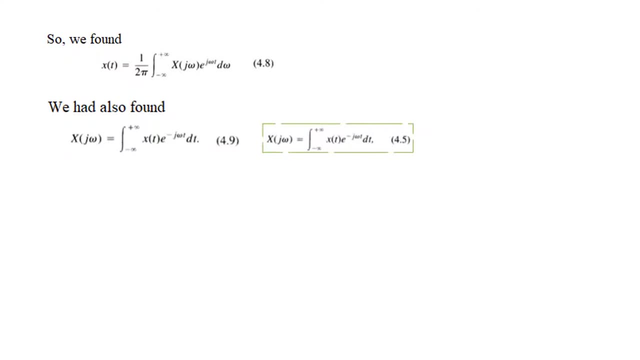 So we have now xt to be in this form, which is equation 4.9.. So capital, X j omega And these two equations are called the Fourier transform pair, Whereas the first one is the inverse Fourier transform And X j omega is the Fourier transform. 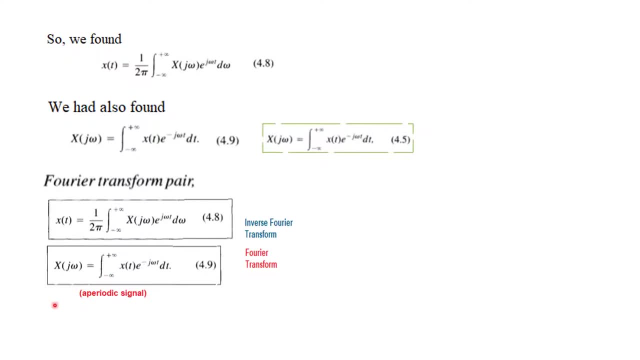 And obviously the transform is for a periodic signal. So this is Fourier transform pair. Now, just for comparison, if you see, in the case of a continuous time periodic signal we had found Fourier series, which was given by this equation. 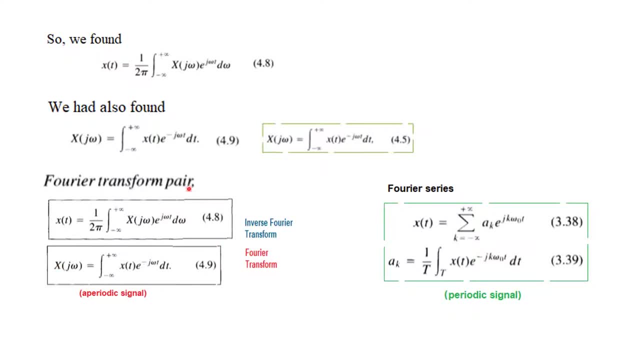 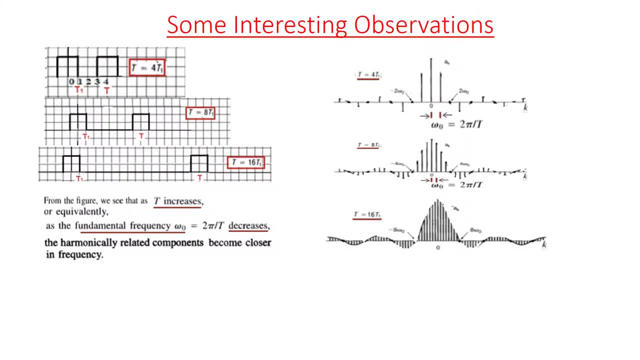 So this is the outcome that we got from our discussion, And now we will use these to solve our problems. Now, having derived the formulas for Fourier transform, let's observe one or two very interesting phenomena. You see, we have drawn three set of graphs or curves. 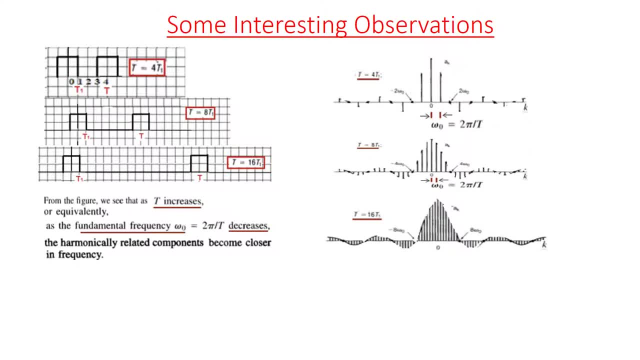 And the difference between the pulses are shown here. So in the first case the difference between two pulse is 41. That is the t, or the time period, is 4 times 4t1.. And for this we have the Fourier coefficient plotted as shown here. 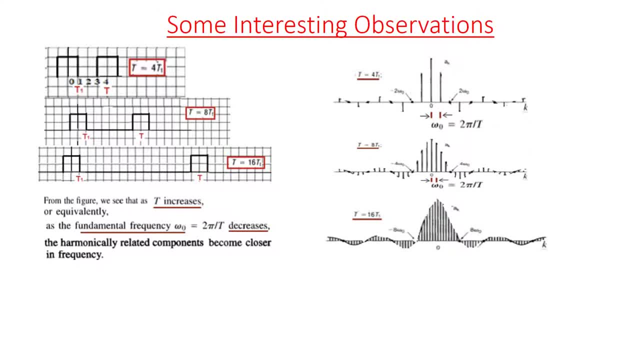 And note that the fundamental frequency omega is 2pi over. t is the distance between any two pulse or any two coefficients. Now, as we are increasing the distance now, this one is now 8 times instead of 4 times. 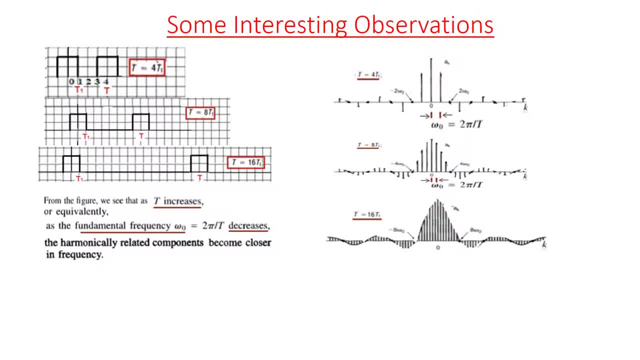 So double the. So this one is now 8 times and this one is now 8 times. So in this case, now you can see that the distance between two amplitudes have reduced. So omega naught is: 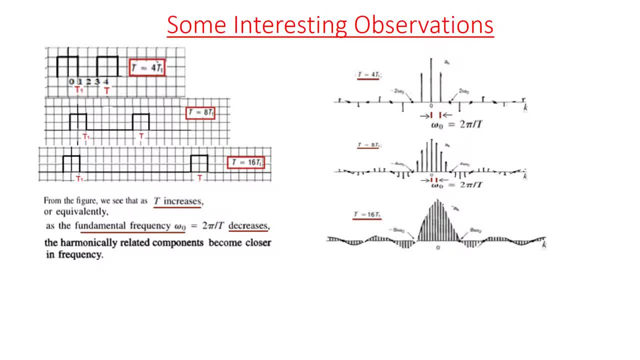 This one is larger and this one is reduced. And in the third case, when the t is 4 times- Sorry, 16 times t1,, then you can see that the impulses or the amplitudes are even closer, Very, very close. 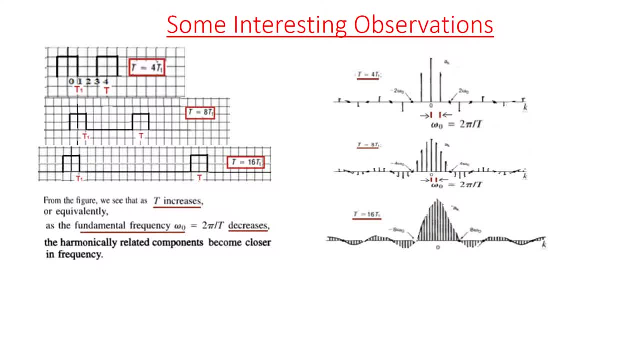 So from this phenomena we can conclude that as t increases or as the frequency decreases, omega naught decreases, the harmonically related components become closer in frequency. So all these components are the harmonic components. This is the DC component. 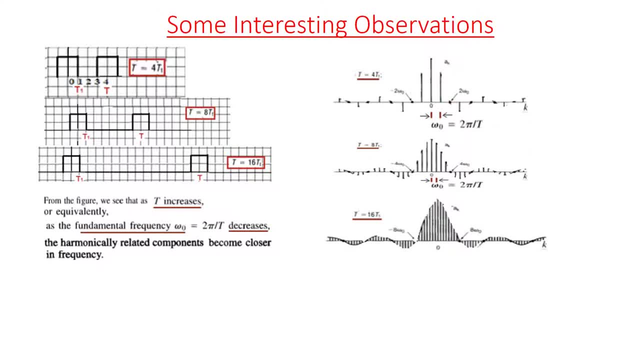 This is the first harmonic, second harmonic, third harmonic. So as As t is increasing they are coming closer and closer and closer, And if we increase this t to infinity it becomes Goes beyond infinity. The next pulse goes beyond infinity. then it will be further closer. 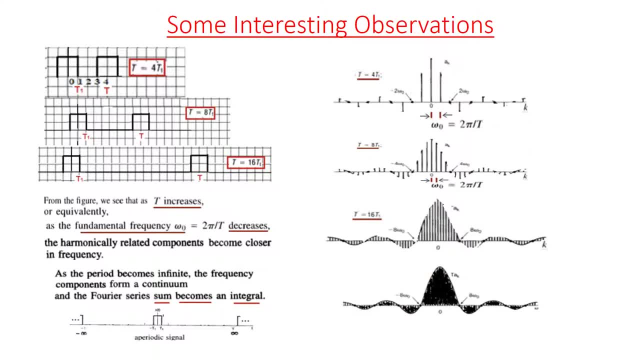 It will be like one unit, one piece, And so in this case Now. So now we are going to see that the summation will become integral, which we had already seen mathematically. Now we are seeing this graphically: how this summation is changed into integral. 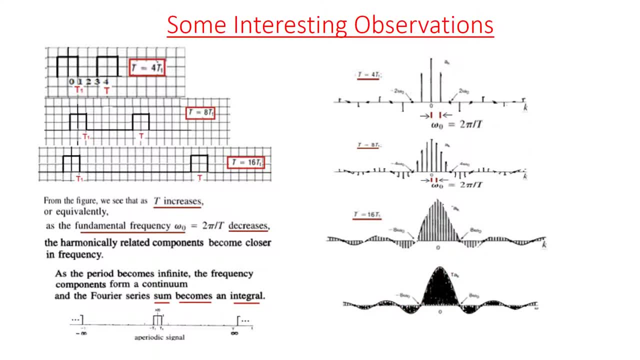 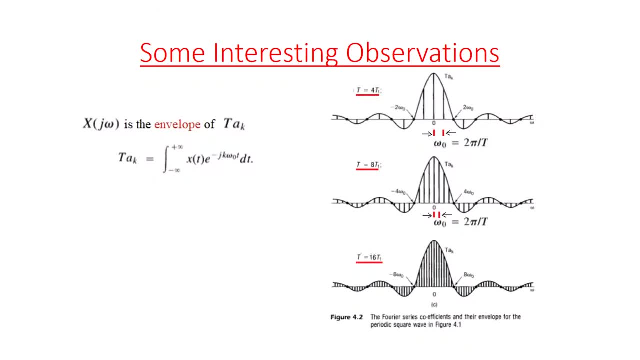 So to find the area or to find the curve, we have to take help of the integral in this case. This phenomena is that we learned that Xj omega is the envelope of Tak. And if you see the equation, The equation, the equation of T a k, this does not have the time period T in it, capital T, that 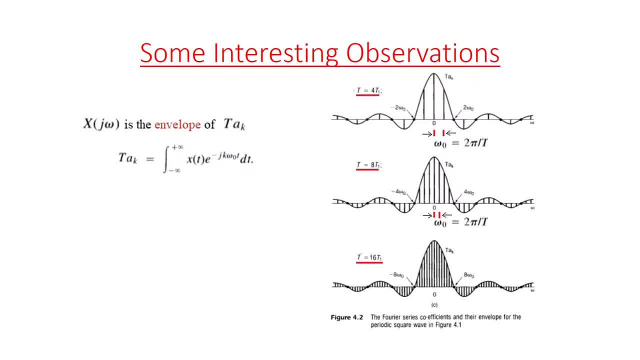 means the T, a, k or the envelope X, J, Omega is independent of the time period T and that you can see from here. and this case T is 4 times T 1, in this case T is 8 times T 1 and in this case T is 16 times T 1, but the shape of the 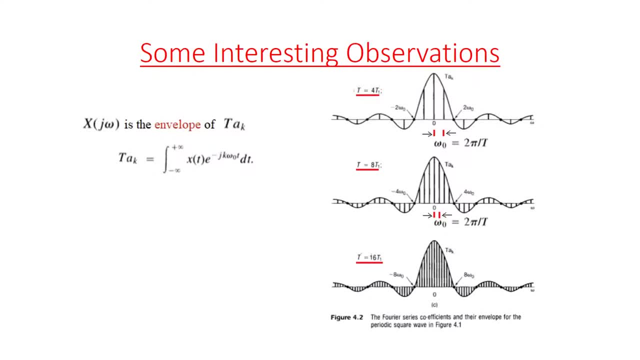 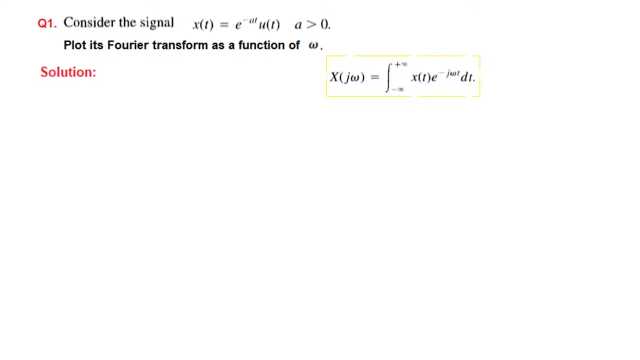 envelope is same, although the amplitudes are coming closer, but the shape remains same, and that is concluded from here that the shape of the curve or the envelope is independent of the time period T. okay, so let's solve the problem. we have the signal given in this form for a 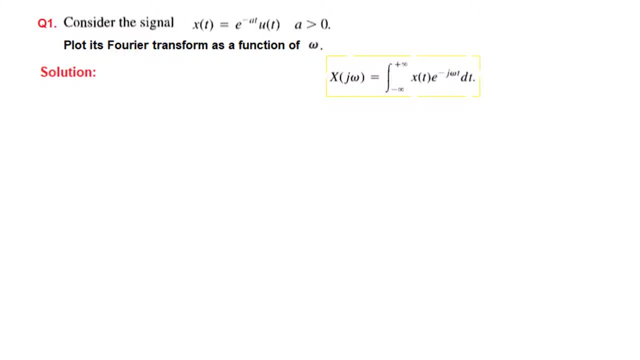 greater than zero, you need to plot the Fourier transform as a function of Omega. now, this was the formula for Fourier transform that we derived. we will use this formula. so now, two things we are doing. number one for X, T, we are putting in the value of E 80, since this is also 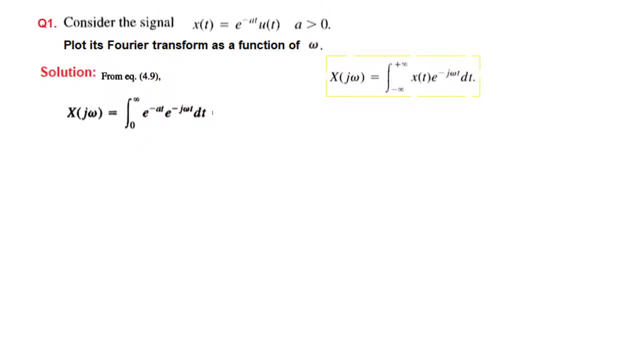 multiplied by a unit function, and we know that unit function is 0 from minus infinity to 0 and is 1 from 0 to plus infinity. therefore, this minus infinity to 0, it will vanish and our limit will start from from zero to infinity. so e a t multiplied by e, j, omega, t, d, t, and we will now solve this. 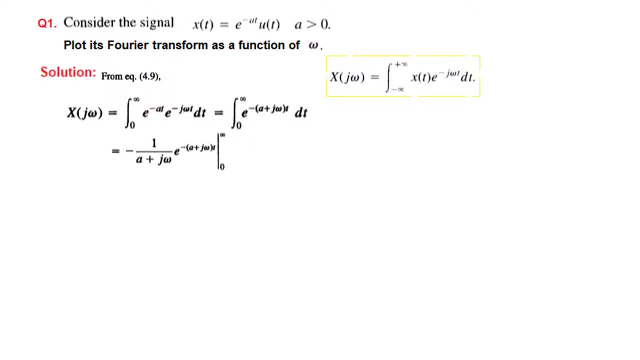 so adding the two powers and integrating. i hope you know how to integrate e power, something t, so it is one over a, j, omega, the minus sign, and this term remains here now putting the limit. i hope you can do this also when we put infinity, t is equal to infinity then, since, 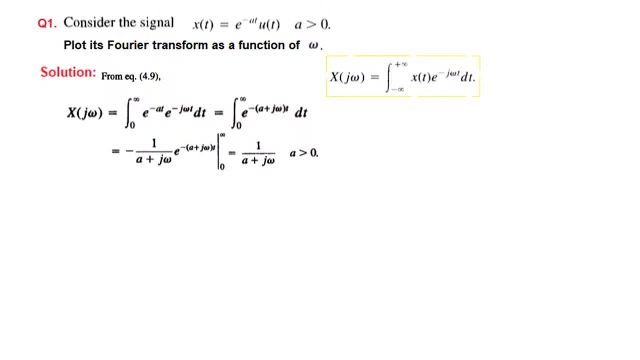 it is e raise to the power negative, so this term will become actually one over e raise to the power infinity, which is equal to zero, and when we put t is equal to zero, this will become one, but after minus. so minus, minus will become plus, and that is why we get one divided by a plus j, omega for a greater than. 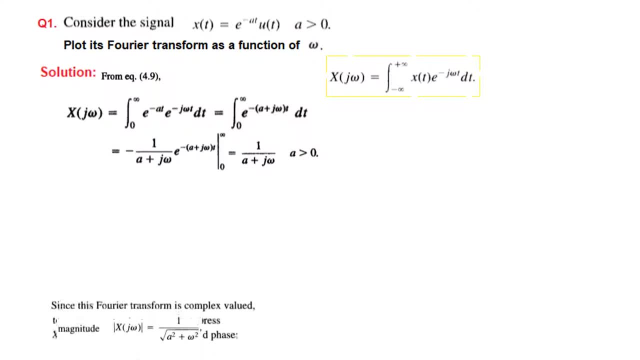 zero. now say, the fourier transform is complex, valued, the plot to plot it is as a function of omega. we express x, j, omega in terms of magnitude and phase. so there will be two plot, one for magnitude and other for phase. this is in complex form, so the magnitude 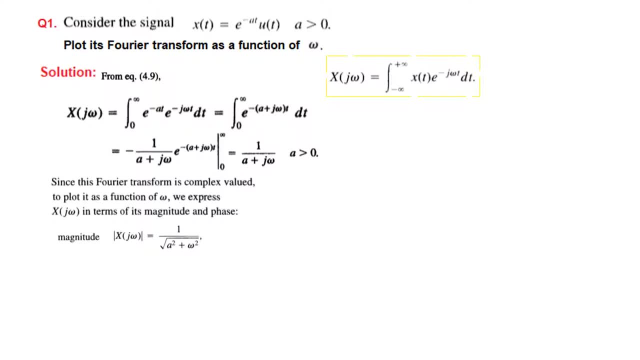 of this, or the magnitude of x, j, omega is, as you know, that square of the two and under root. so this is the magnitude. and to plot this magnitude we take one or two values. first of all, at omega is equal to zero, this will become one over a. similarly, at, omega is equal to plus minus one, plus minus a, as j, omega will become one over and the root two a. or this can also be written as if you multiply under root, on both sides: under root two divided by two a. 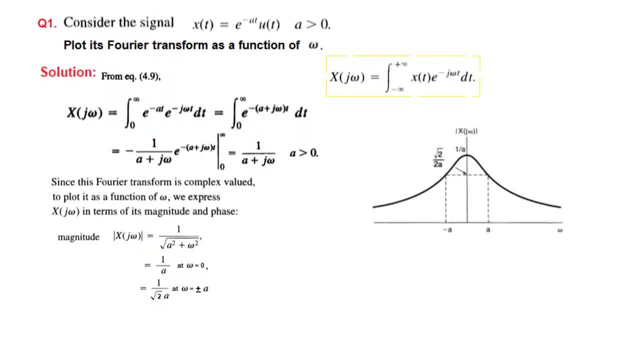 This is shown in this plot: At omega is equal to 0, at omega is equal to 0, it is 1 over alpha, So the value is 1 over alpha And at omega is equal to a plus minus a the value. 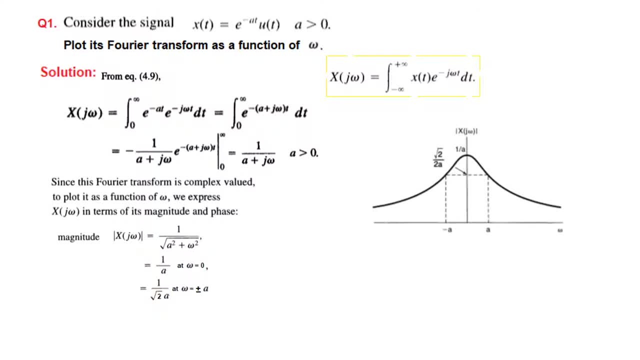 is 1 over under root 2 a. Or, as I told you, that if you multiply numerator and denominator by under root 2, then it will become under root 2 divided by 2 a. So these are the two points And if you take couple of more points you will get the exact shape of this curve. 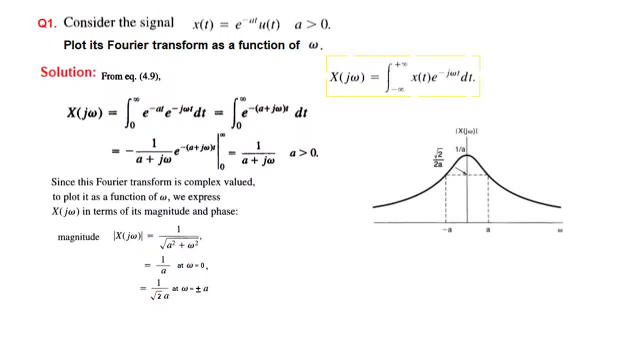 So this is representing the magnitude term. Now we come to the phase term. So from here I hope you know how to find the phase angle: minus tangent omega over a. So minus tangent inverse Omega over a. If you have difficulty, you have got to revisit the earlier part of the. 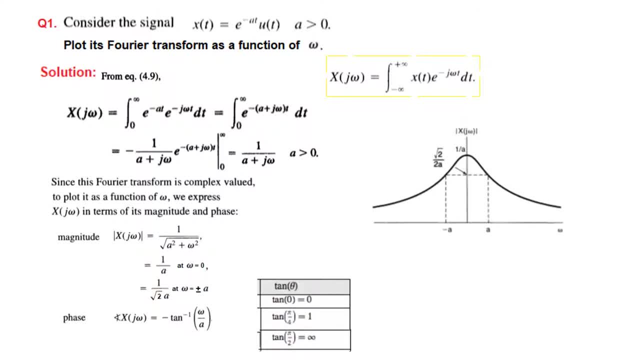 circuit analysis. And now we know from the values of tangent that when angle is 0, tangent is 0. At angle pi by 4, its value is 1.. And at pi by 2, its value is infinity. So this: 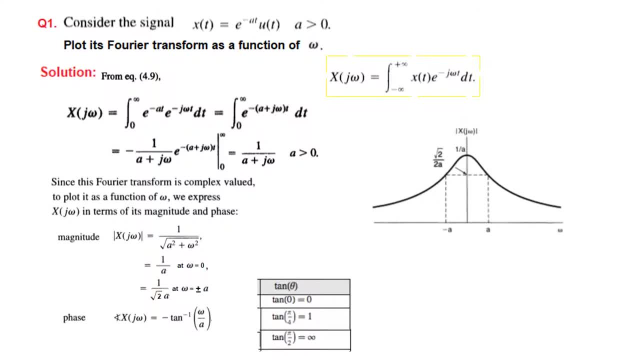 is the tangent. So from here we can take the tangent inverse. Let us see Now: at omega is equal to 0.. At omega is equal to 0, this will become 0. So tangent 0 is 0.. So this: 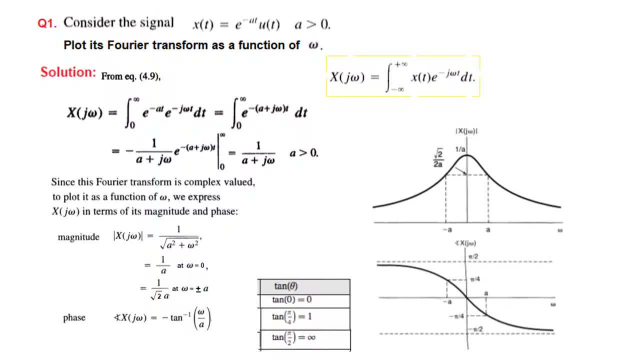 is the plot is here At: omega is equal to a, this will become a divided by 2.. So this will become a divided by a1.. And from here you can see that if you take the tangent on the right hand side, So tangent inverse a is pi by 4.. So it is at plus pi by 4 and 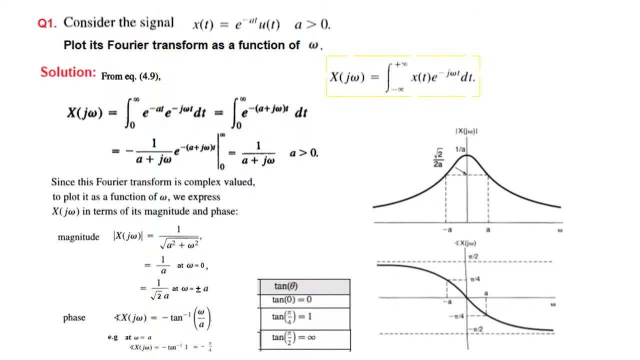 at minus pi by 4.. And similarly, if omega is infinity, So tangent infinity or tangent inverse infinity is pi by 2.. So at pi by 2, it is going towards the infinite limit. Omega is infinity. So this is how you. 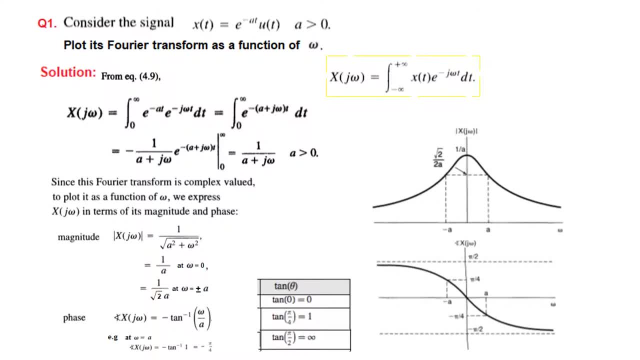 can plot the phase angles. I hope this video gives you some idea about the Fourier transform, So if it helped you, please subscribe my channel. Thank you.